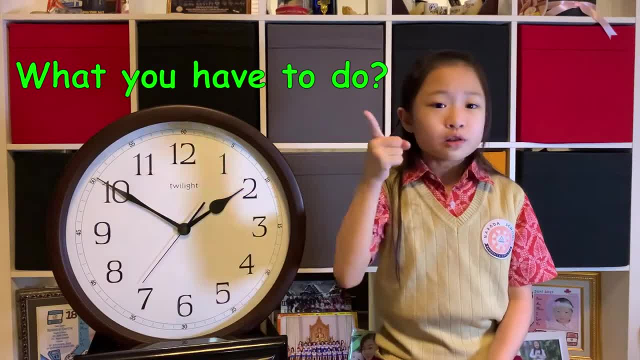 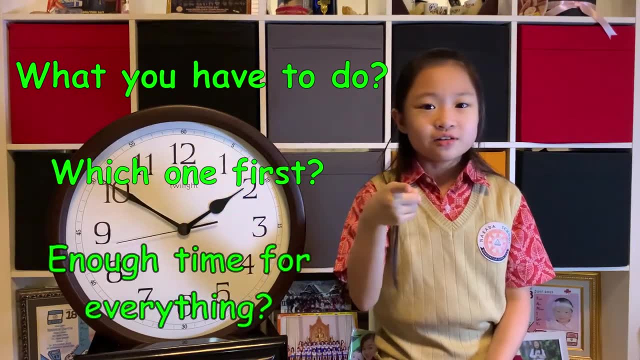 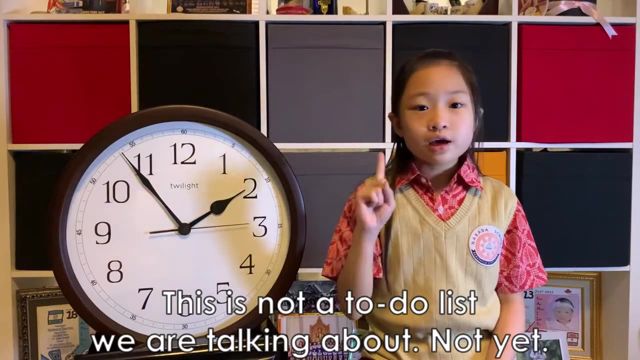 But how do you spend that 24 hours per day? What do you have to do? Which one first? Enough time for everything. Let's break it down. First, list down your tasks. This is not a to-do list we're talking about Not yet. 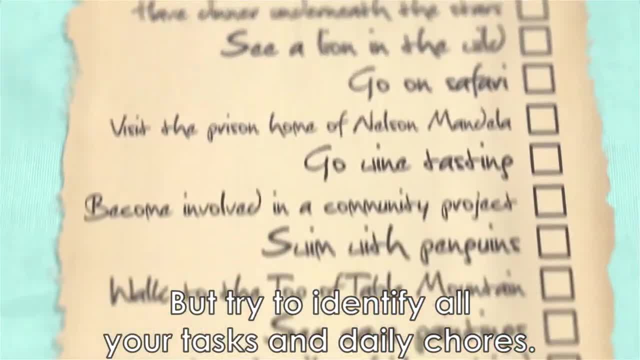 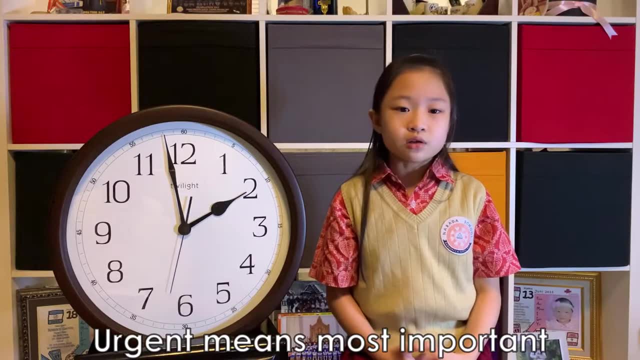 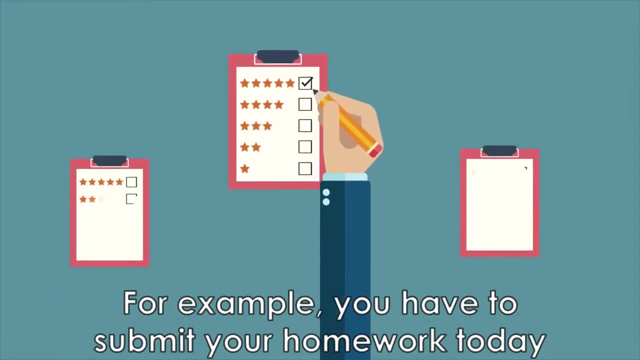 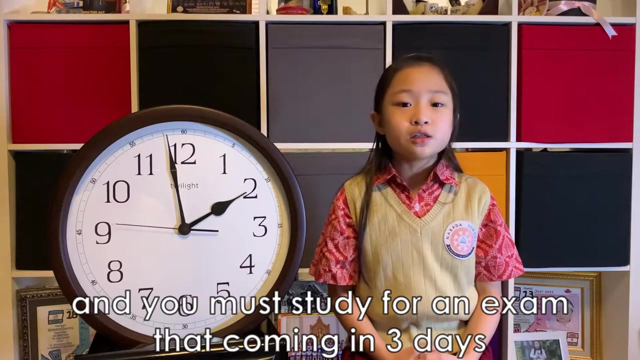 But try to identify all your tasks and daily chores, List it down Which one is urgent. Urgent means most important. Pick the important tasks from your list and finish it first. For example, you have to submit your homework today and you must study for an exam that's coming in 3 days. 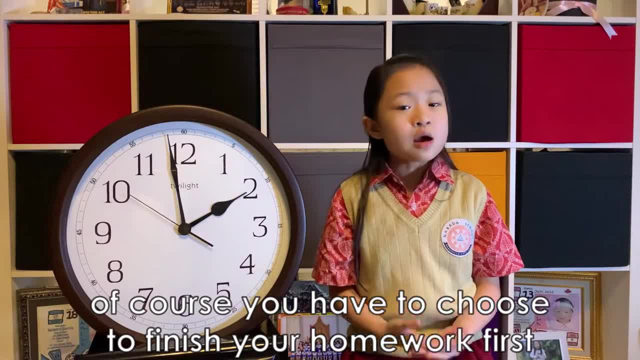 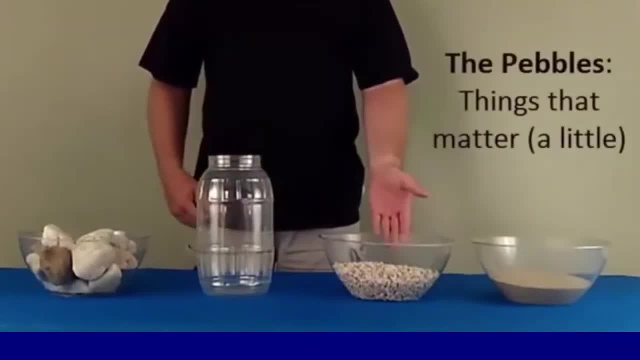 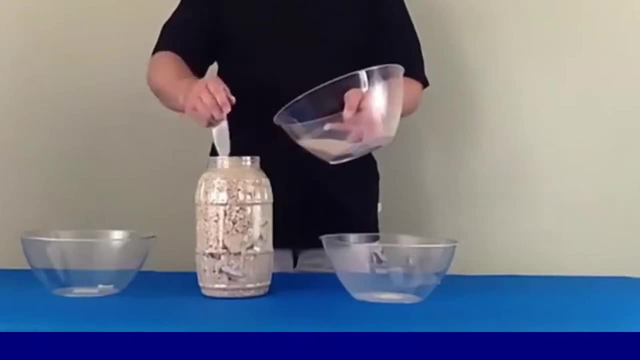 Of course you have to choose to finish your homework first Before studying for the exam. it is like how to fill a jar with big stones, pebbles and sand. Always put the big thing in first and the next smaller, and so on up to sand. 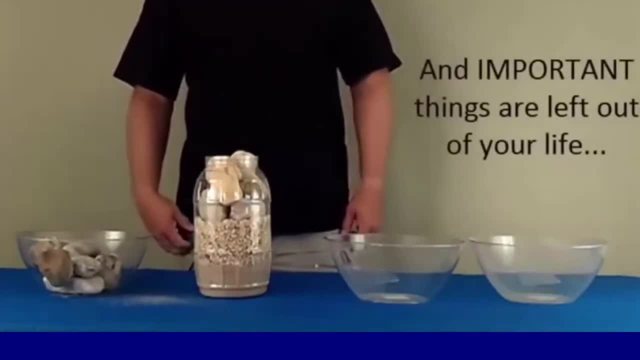 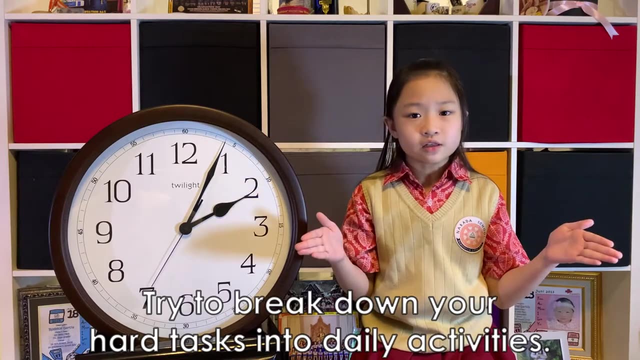 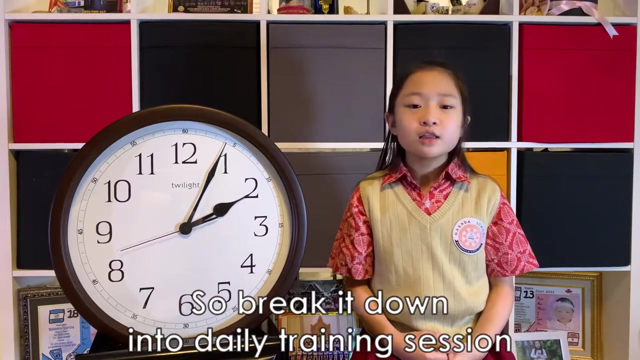 You will fail if you fill in small things like sand. first, Daily activities: Try to break down your hard tasks into daily activities. For example, you cannot master a piano in 24 hours. It needs time. So break it down into daily training session. 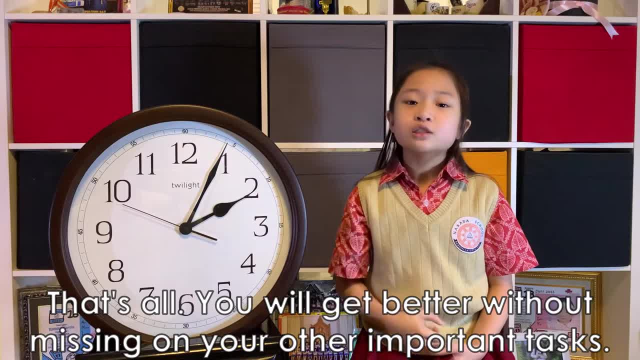 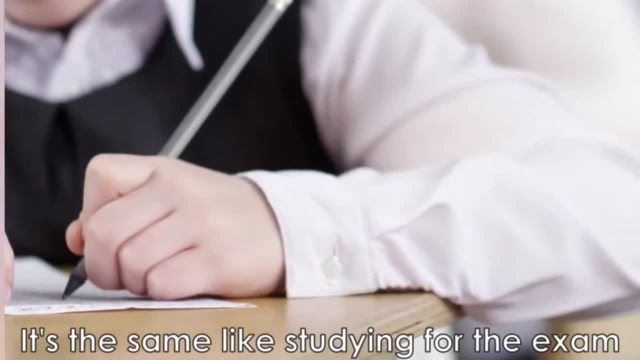 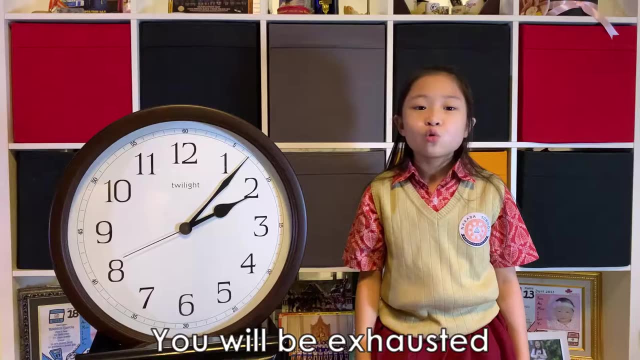 20 to 30 minutes a day. That's all You will get better without missing on your other important tasks. It's same like studying for the exam. You don't have to study all day. on the exam day, You will be exhausted and most likely forgot what you learned about. 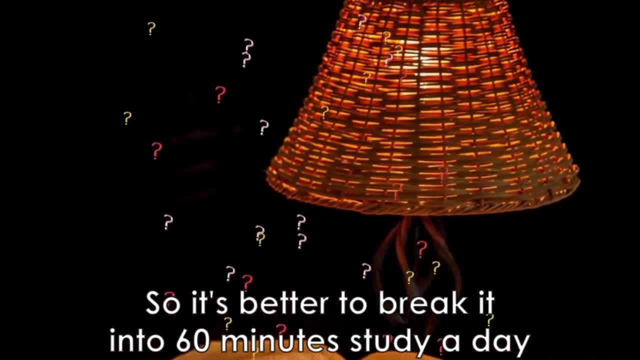 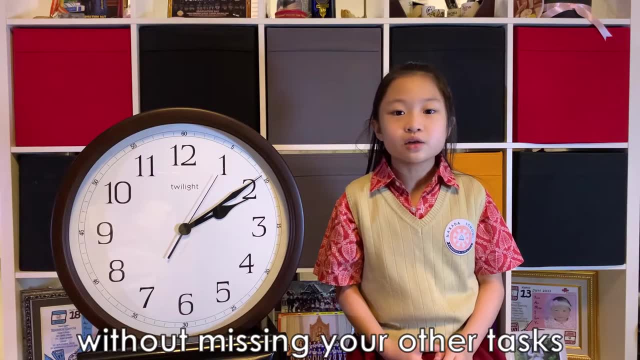 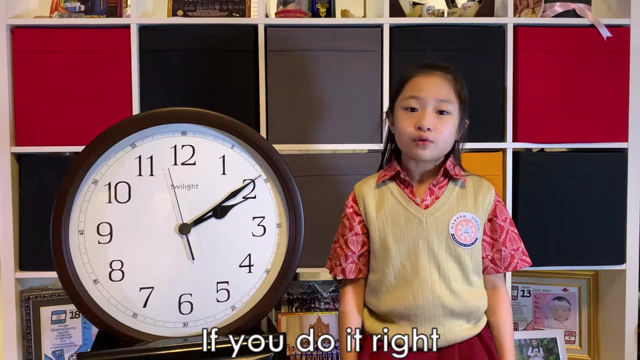 So it is better to break it into 6 parts: 60 minutes study a day. Do it 7 to 10 days before the exam. You will do much better without missing your other tasks. You can still rest and play too. Have fun. If you do it right, then it will make your days much more enjoyable Being